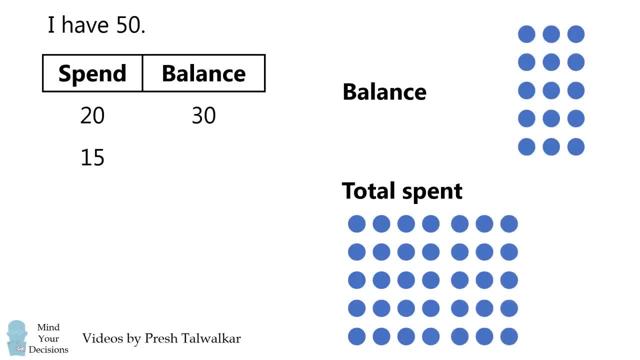 Well, what happens if we spend 15?? We then remove 15, and we have a balance of 15.. So far, so good. Now we spend 9,, which leaves a balance of 6.. And then we spend that 6, and, of course, we're going to have a balance of 0. 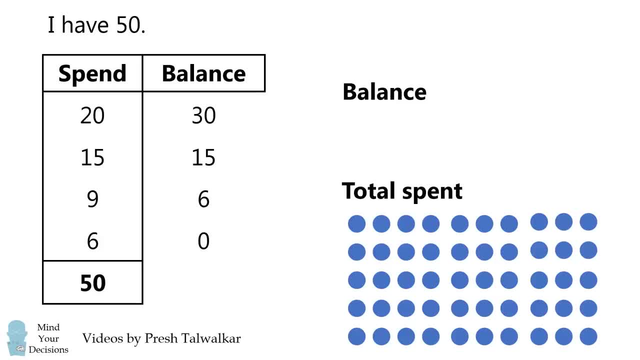 So actually all of these numbers are correct, The total amount that we spend will be equal to 50. The question is, why is the total in this balance column equal to 51?? Well, the reason is there's actually no problem with the numbers. 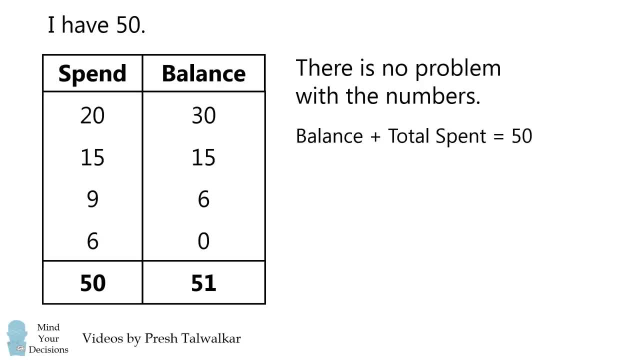 The correct equation is that the balance plus the total amount spent will be equal to 50. It's not going to be true that the sum of the balance column will be equal to 50. Sometimes it will be, but in this case it'll be equal to 51.. 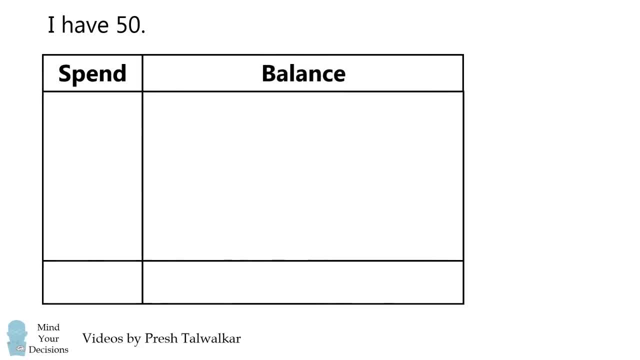 Let's think about this problem a little bit more abstractly. Let's suppose we spend S1. Our balance will be 50 minus S1. If we then spend S2, we have a balance of 50 minus S1, minus S2.. 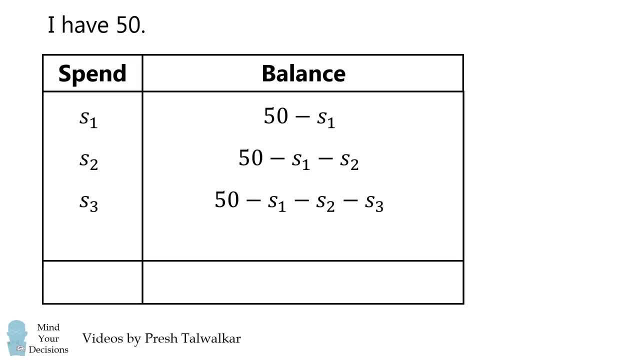 If we then spend S3, we subtract S3 from the balance column. We then have S4 and subtract that. The total amount in the spending column will be the sum of these spending amounts And now the total amount in the balance column will be this function. 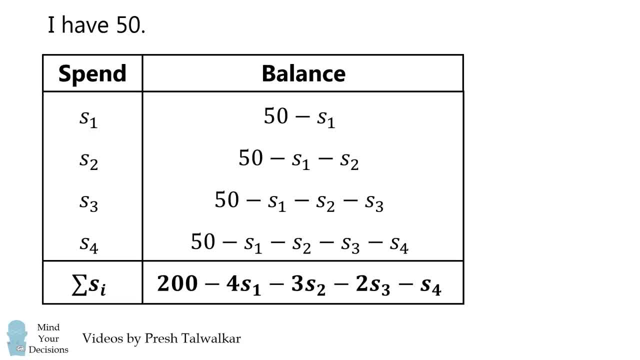 200 minus 51.. 200 minus 4 times S1, minus 3 times S2, minus 2 times S3 minus S4.. If we put in the amounts from the original problem, we can see what the result is for each of these columns. 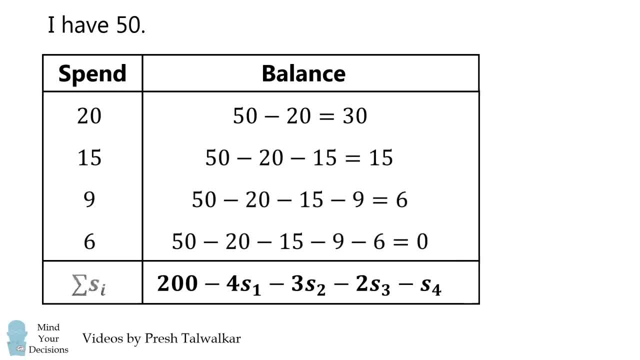 So all of these numbers will actually be correct. The total amount in the spending column will be 50.. But now the balance column. when we evaluate this function, we get a result of 51.. And that's fine. It doesn't have to be equal to 50. 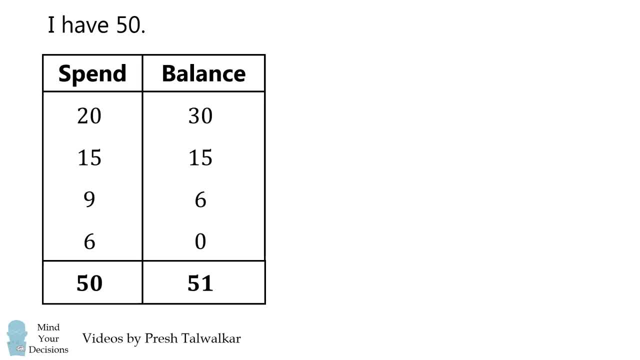 So if we go back to the original problem, we get a result of 51. But if we go back to the original table, it's completely correct and there's no problem with the numbers. It's just a trick question to compare the sum of these two columns.